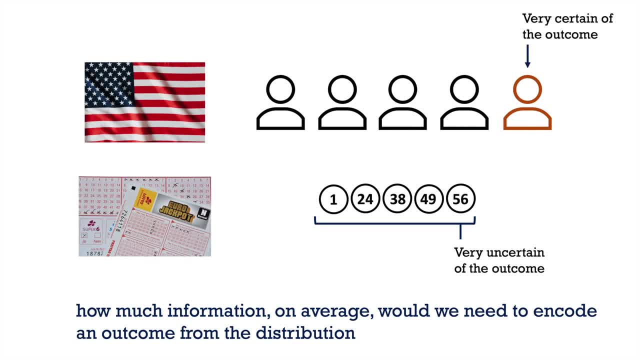 actually happened, But if the outcome is effectively known beforehand, then you'll need little information, maybe even none, to know the outcome. This idea of information may be confusing, so let's introduce a setup that may explain what we mean by this. 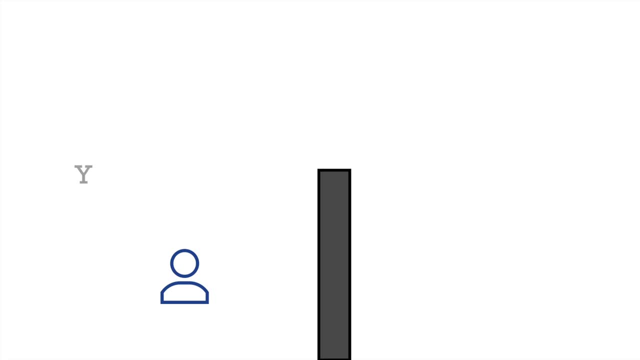 Imagine that we are on one side of a wall where a random outcome occurs. The outcome is drawn from some underlying random probability distribution. We can observe the outcome of the event. however, there's another person on the other side of the wall who cannot observe the outcome. Our goal is to let the other person know the outcome of. 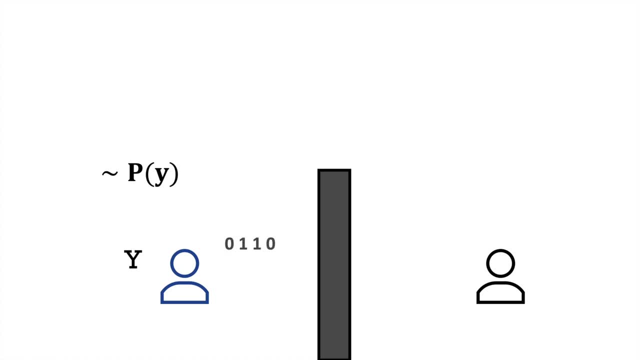 the event by only sending a single n-bit number across the channel. Note that before the experiment, we can agree on a mapping function of bits to some real event. However, once we cross the wall, we can only send the n-bit number across the channel. 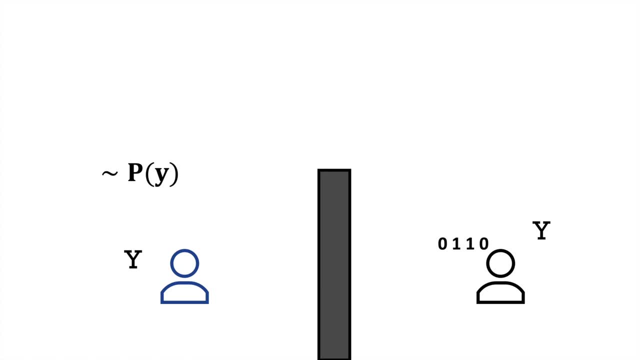 In this setup, the n-bit number is the information. For example, let's assume that the random event is a coin flip. We know that this probability distribution only has two equally likely outcomes: heads or tails. Hence we will only need a single. 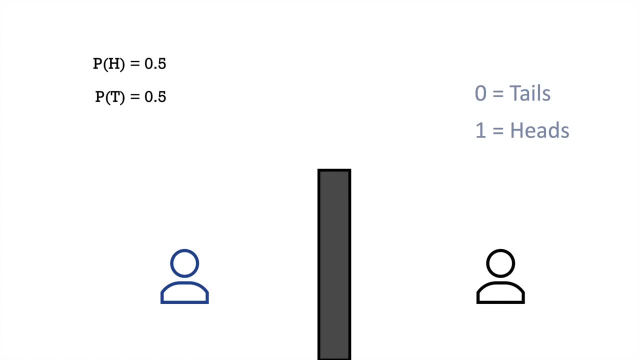 one-bit number to describe the outcome. Zero can map to tails and one to heads. After observing the outcome of the coin flip, we can send the relevant bit across the channel to the other person and they will know exactly what the original observation was. So this coin. 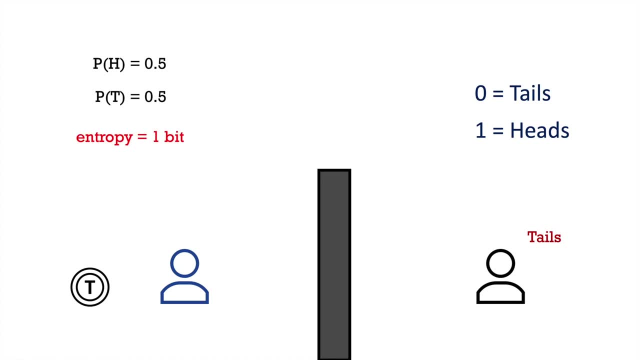 distribution has an entropy of one bit, ie it only takes one bit of information to entirely describe the outcome of the event. Now imagine a similar random event, but now with eight different possible outcomes. Maybe there's an international football tournament with eight equally strong. 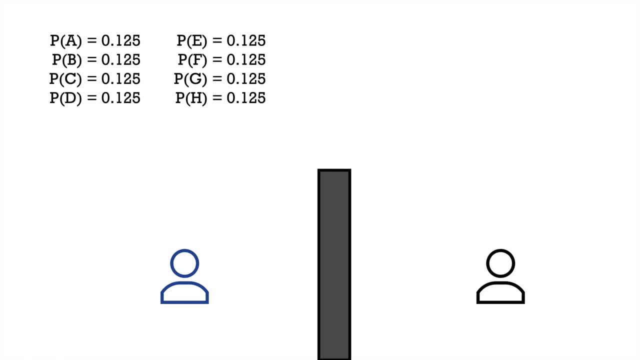 teams, so the probability of any team winning the tournament is one over eight. In this case, we now need three bits to encode the outcome, as three bits can describe two to the power of three, which equals eight different states. So, after observing which team won the 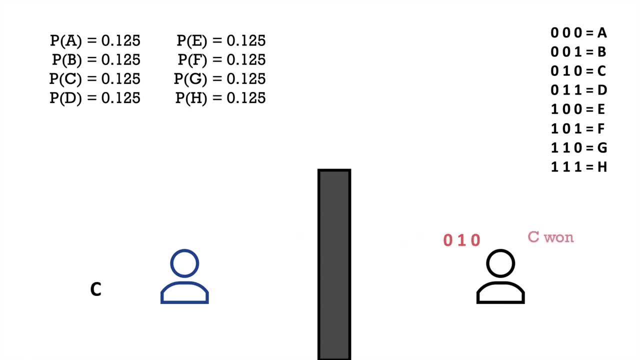 tournament. we can send a three-bit number to the other person and they will know exactly what the outcome was. Therefore, this distribution has an entropy of three bits. Hopefully we can see that this argument could generalize further to distributions with different number of outcomes. 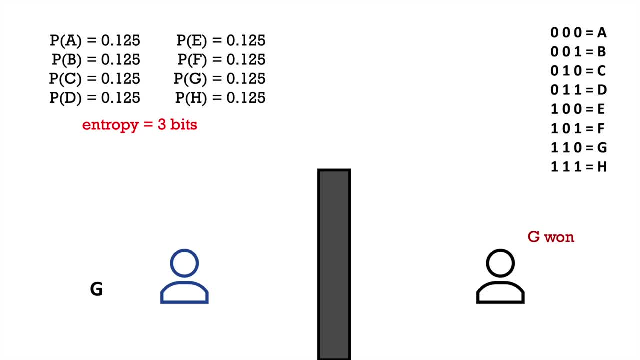 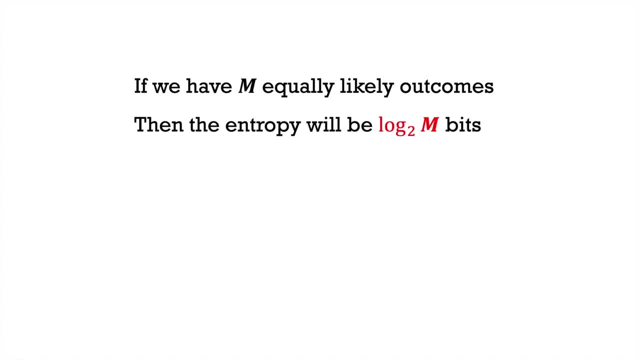 In fact, for a uniform distribution with m possible outcomes, we could write the number of bits required as log base. two of m For powers of two. this is trivial to see. Log base two of two to the n is n and n bits allows us to encode two to the n different states, showing us that this formula. 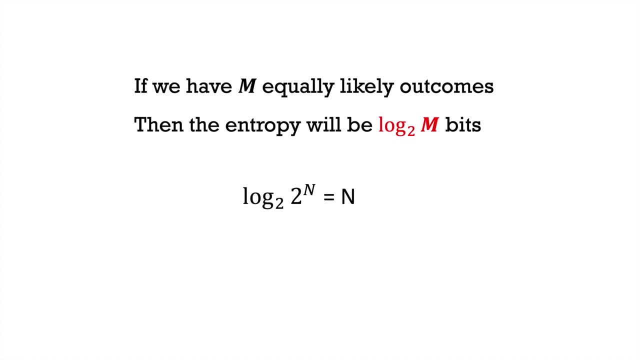 works. However, we can also show that this formula even holds for uniform distributions where the number of outcomes is not a power of two. Let's show this for the case where m equals ten. Assume that we have a distribution with ten equally likely outcomes. Four bits give sixteen. 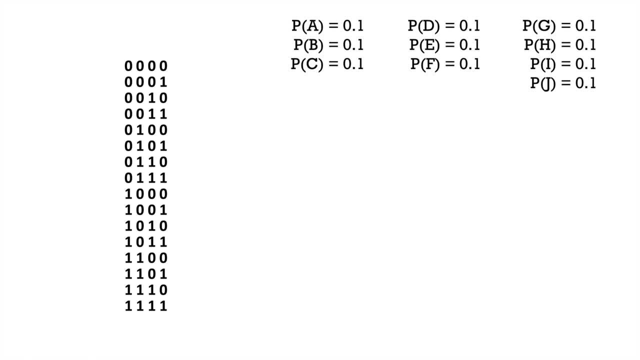 unique states, so we could in theory, use four bits to encode every possible outcome. However, this is inefficient as it leaves six states left over. To do better, we can observe three separate outcomes and encode the outcomes in groups of three. Each outcome can be one of ten. 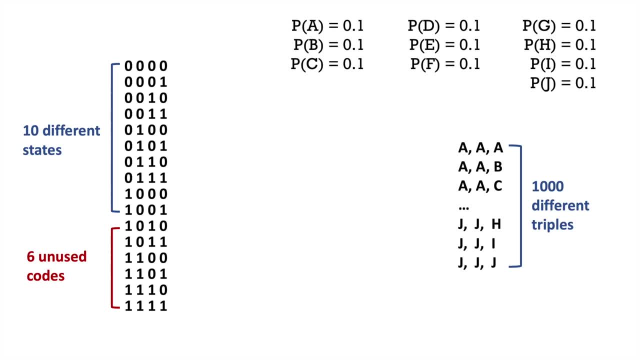 different states. so there are one thousand different possible triples of outcomes. Ten bits will give us one thousand and twenty-four different states, as two to the ten equals one thousand and twenty-four, which is sufficient to encode all one thousand unique states. So what we're saying? 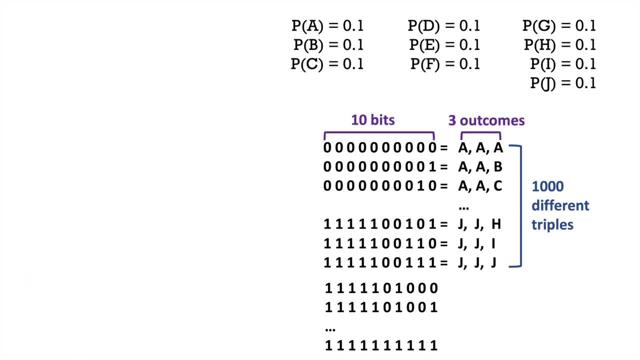 is that, with ten bits, we can encode three independent outcomes. The average number of bits per outcome is then ten divided by three, which equals three point three, three, three. This scheme, though, isn't completely efficient, as we still have twenty-four unused states. 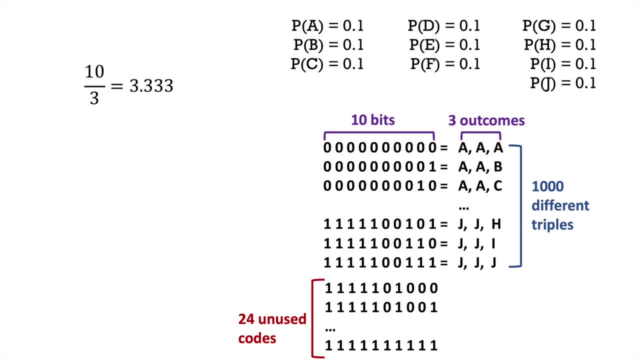 For the most efficient encoding scheme. we're looking for the case where ten to the g equals two to the b, where g is the number of grouped observations. By taking the log of both sides and rearranging we can show that the most efficient number of bits 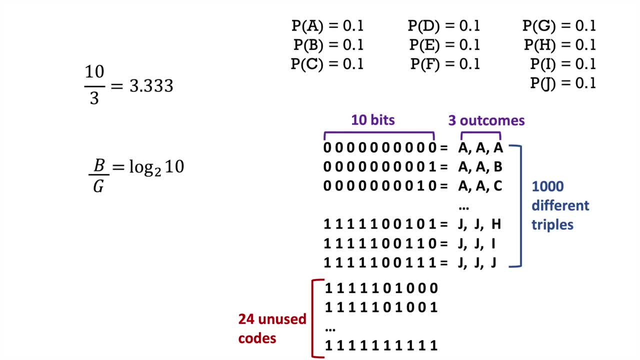 to encode each outcome is log base two of ten, which is the entropy expression. Also, log base two of ten is three point three, two, which is very similar to our three point three, three, three estimate. Let's return back to the discussion of entropy. We've shown that for a 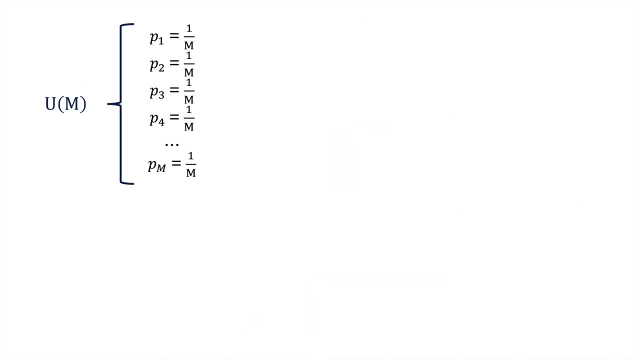 uniform distribution with m outcomes. we can encode a number of bits per outcome, which is two to the g. The entropy is log base two of m bits. However, there still is a big issue, which is that most distributions are not uniform. That being said, we can use our previous statement to help measure the 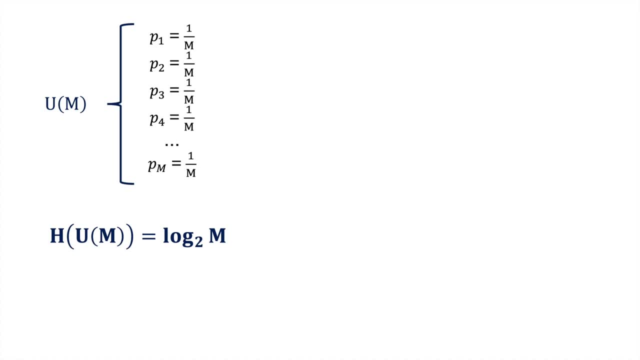 entropy of any distribution, even non-uniform ones. We do this by associating bits to outcomes. A m-uniform distribution has m possible outcomes, each with probability one over m. So, in terms of entropy, we can interpret each outcome as a number of bits per outcome, which is two to the g. This 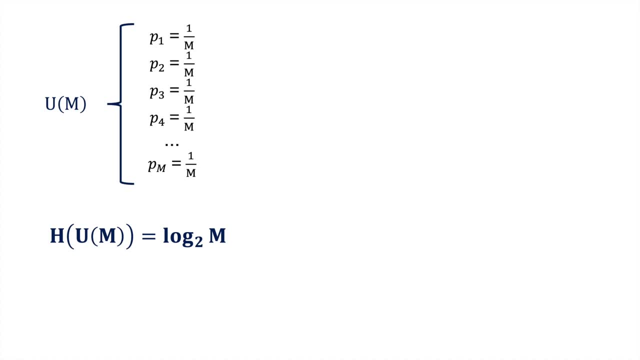 can be simplified by taking the fraction out. Note that if we plug in the probability of one over m in, we get the expected expression of log base two of m. For an arbitrary probability distribution. where the probabilities vary, we can say that if an outcome has probability of pi, 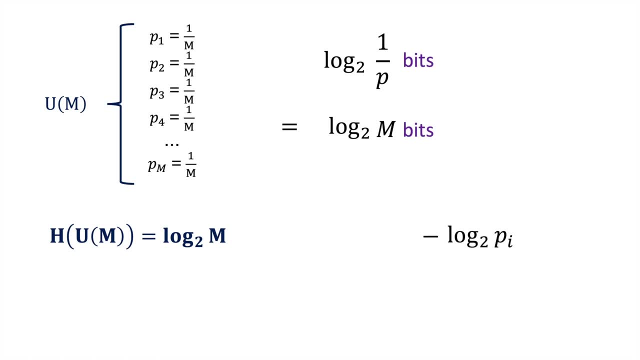 then this many bits are needed to encode that outcome And we can calculate the expected number of bits over all the outcomes by multiplying the expected number of bits per outcome. We can also calculate the expected number of bits over all the outcomes by multiplying the expression by. 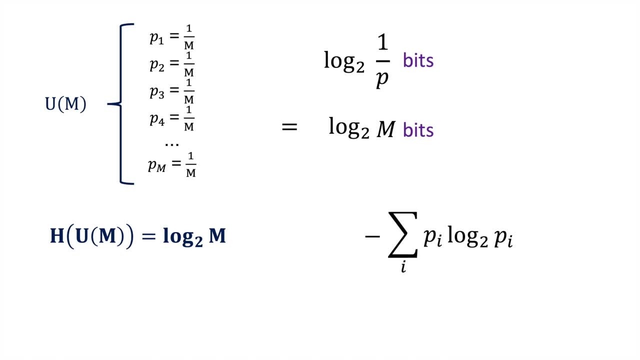 each probability and summing over all possible events, This leads to an expression which may look familiar, as this is the Shannon entropy formula. So this is my interpretation of the Shannon entropy formula. It is the measure of how much information, on average, is needed to 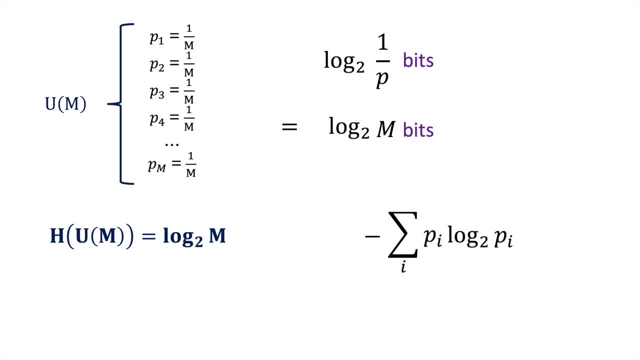 describe outcomes of a distribution. It is linked tightly with uncertainty, since if we're less certain of an outcome, we may need more information to describe it. Why is entropy important? Well, it's because it can provide useful statistics for how much information we gain from observing an outcome. 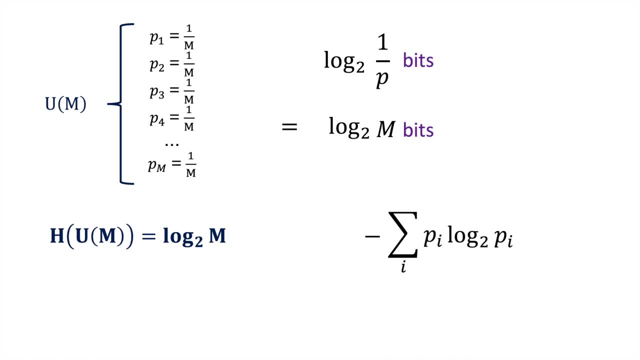 or tell us how varied the outcomes of a distribution are. As a result, this expression crops up in many places, particularly within information theory. This marks the end of the video. Hopefully the content helped you understand the Shannon entropy a bit better and gave intuition for how it measures uncertainty. If you want to stay posted, 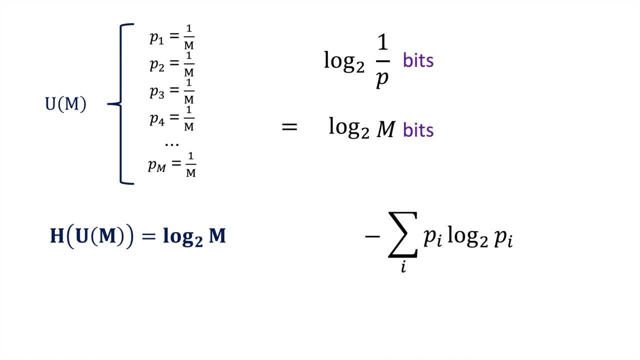 for any probabilistic theory or machine learning content from this channel. then remember to subscribe to get any future videos. Thanks for watching and I'll see you in the next video. I'll see you in the next video.